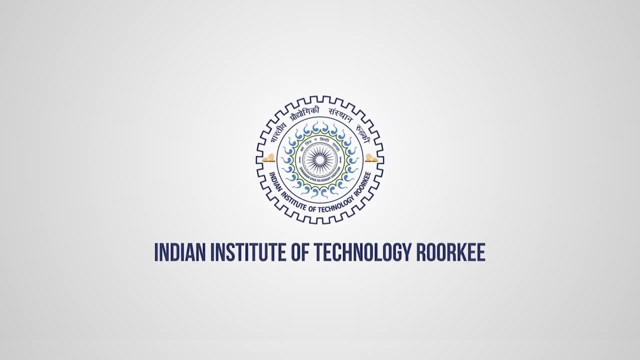 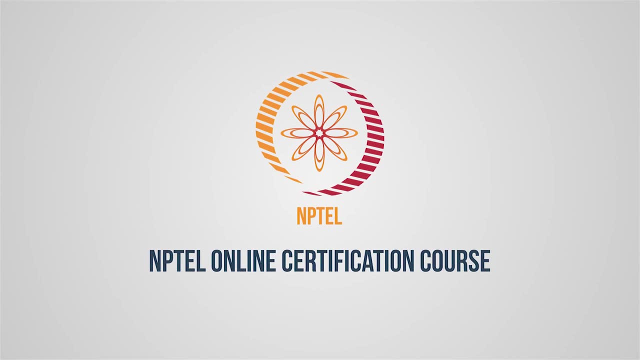 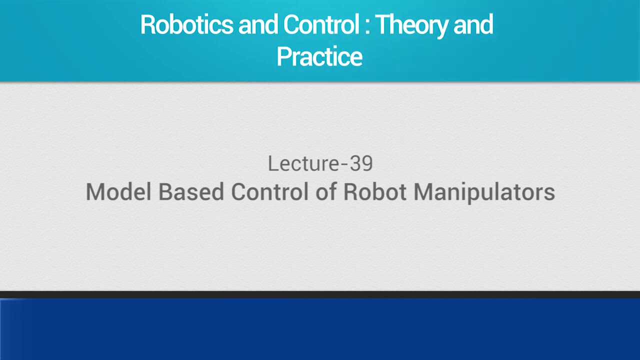 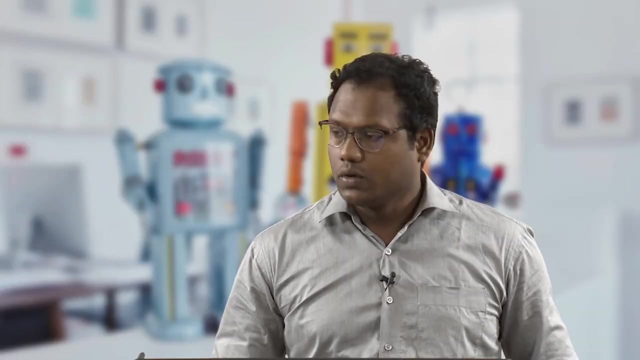 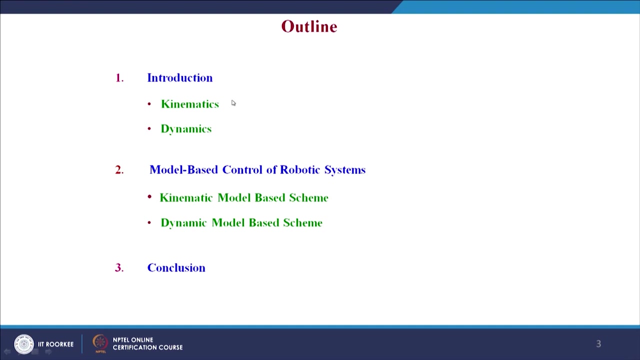 Good morning. Today, we are going to see about model based control of robot manipulators in this lecture. The outline of this lecture will be as follows. First, we have the introduction 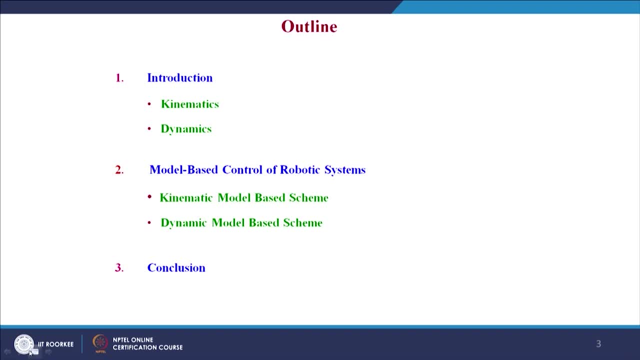 where we will be discussing quickly about kinematics and dynamics kinematics definition dynamics definition what is forward and what is inverse kinematics and what is forward dynamics and what is inverse dynamics and then we come into the major portion which is the model based control of robotic systems. Model based implies both kinematic model based scheme and dynamic model based control scheme and finally, we conclude. Now, coming to the introduction first we talk 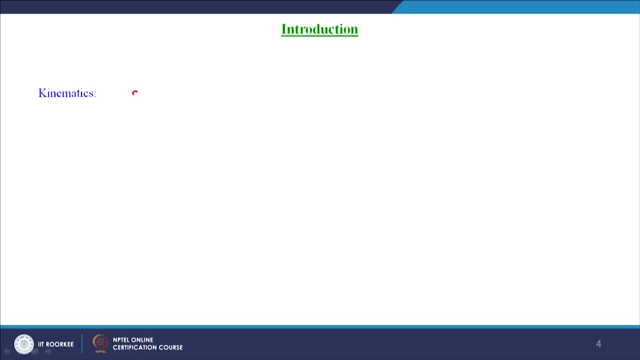 about kinematics. What is kinematics? Kinematics is the study of motion without considering the forces associated with kinematics can be classified the robot kinematics can be classified into forward kinematics which is the input is joint angles whereas, the 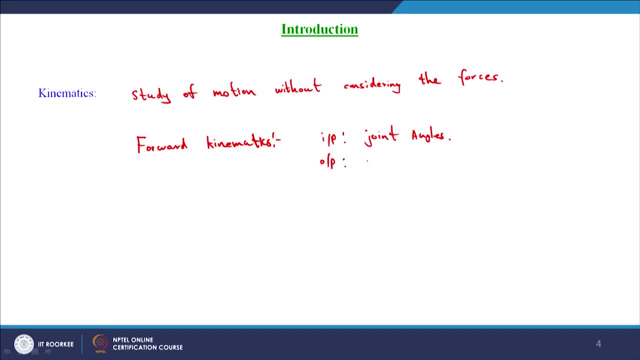 output is end effector force which nothing but position and orientation whereas, inverse kinematics. 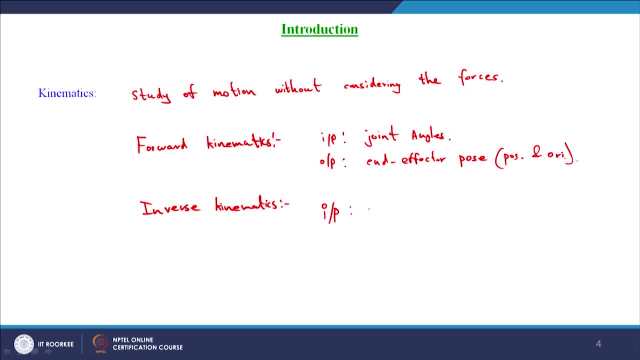 So, input is end effector force and the output is joint angle. Now, coming to the dynamics portion, what is dynamics? Dynamics is the study of motion considering the forces associated with that motion. Dynamics can be further classified into inverse dynamics and forward dynamics. What is inverse dynamics? Inverse dynamics, the input is joint trajectories in terms of theta, theta dot and theta double dot, position, velocity and acceleration of the joint angles. And the output is this is the input is joint trajectory, the output is joint torque. Whereas, for the forward forward dynamics, the input is joint torque, the output is joint trajectories theta, theta dot and theta double dot. The inverse dynamics is useful. 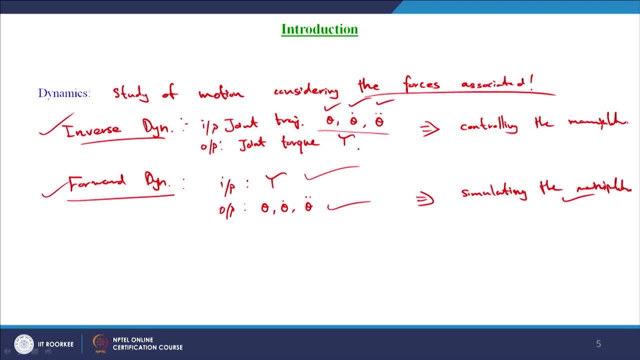 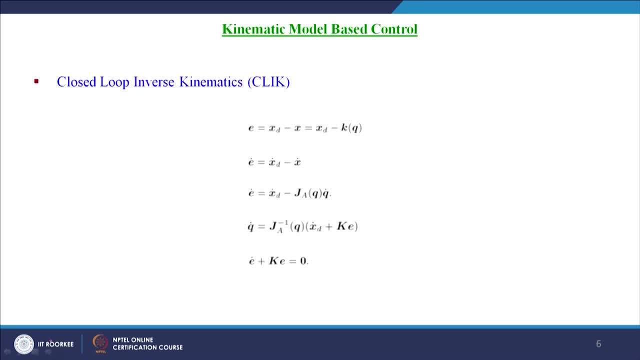 The inverse dynamics is used for simulation of the manipulator and inverse dynamics is meant are used for controlling the manipulator. Now, coming to the control based on the model of the manipulator, thus model based control, first we discuss about kinematic model based control. It is nothing, but closed loop inverse kinematic scheme. . Because, we ensure that the error goes to 0 as the time tends to infinity by a first order dynamic equation. So, CLIK closed loop inverse kinematics algorithm is derived in such a way that, the control law is given by q dot which is the generalized coordinate of the joint is given by q dot. . 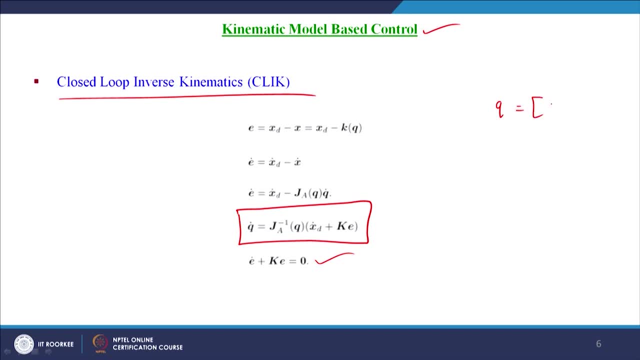 joint is given by q which can take either theta for prismatic joint or d for theta for revolute joint and d for prismatic joint the joint variables. So, generalized joint coordinate can be represented by the letter q. So, the joint velocity is represented by q dot and the control law under this CLIK is given by q dot equal to j inverse which is a function of q multiplied by x d dot plus k e. So, this takes care of the error 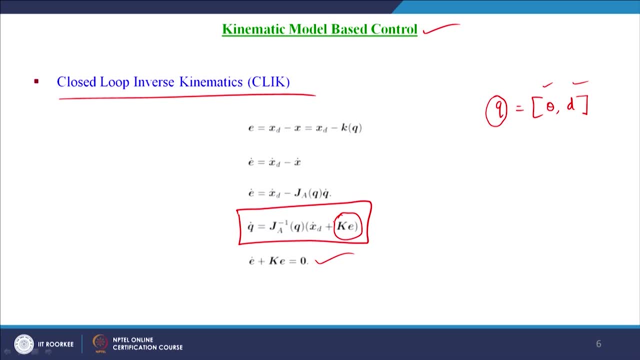 that is associated with the cortisone trajectory. 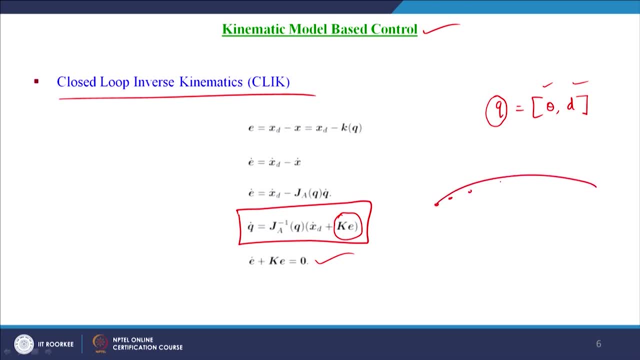 Desire trajectory. Actual. In the inverse kinematics desire trajectory is given in the cortisone space for the tip 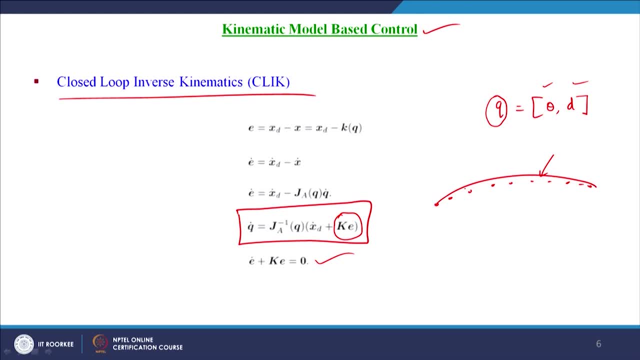 of the manipulator and the actual tip should follow that trajectory by the computation of the joint angles. 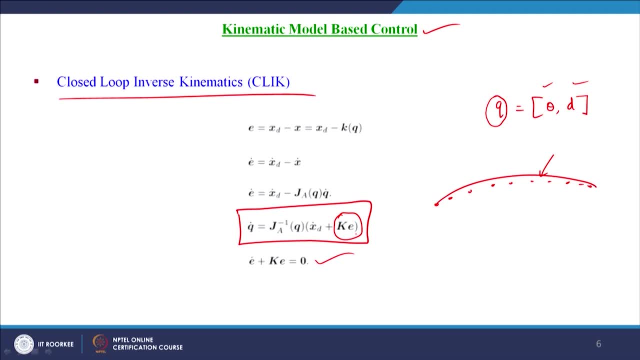 That computation of joint angles is obtained by this control law which takes care of this error getting. Minimized. 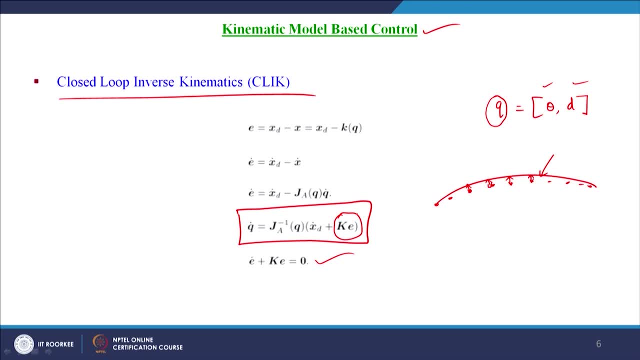 This discrepancy getting minimized is ensured by this control law. 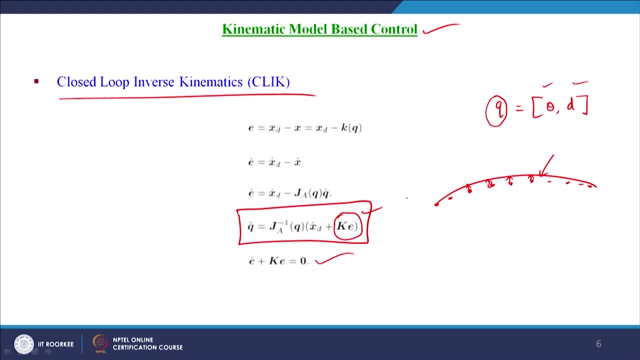 So, the control law how we can derive this which states that first order dynamic error dynamic equation. 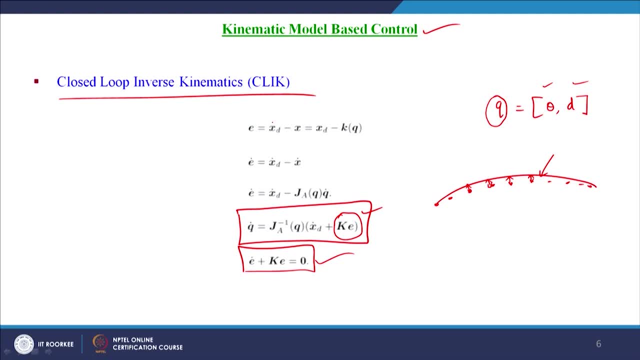 So, the error is given by the discrepancy between the desired trajectory and the actual trajectory. 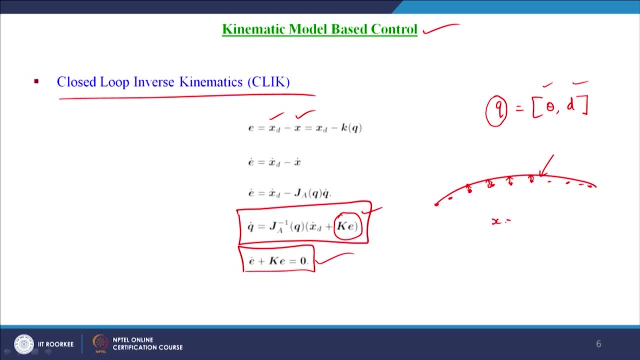 Where the actual trajectory is given by the forward kinematics function of q that is what is represented as k of q here which is nothing but the end married vector position. 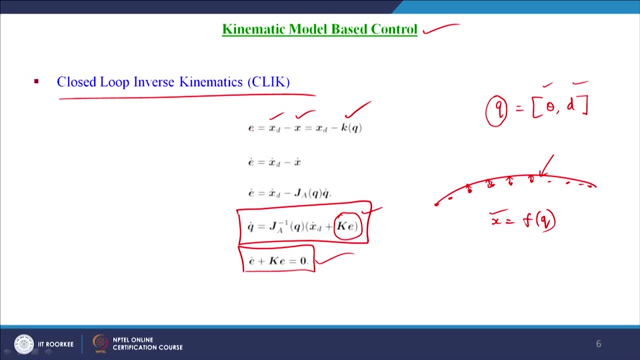 So, error is the difference between the desired trajectory and the actual trajectory and the error dot is the time derivative of the error is e dot equal to x d dot minus x dot. So, Now, x dot is represented by J Jacobin into theta dot we know that from this, this is forward kinematics the differential kinematics is f x dot equal to J q dot that is what is my pushed put here. And from this we have this q dot given by this control law also q dot is given by this control law. So, this. So, when we equate q dot is given by J inverse into x d dot plus k e. So, these two equations, equation 1 and equation 2 both corresponds to both correspond to q dot. So, when we when we equate this we will have e dot which is we will have the x d dot minus x dot plus k e is equal to 0 which is given by e dot plus k e equal to 0. That is what this first order equation is known as the dynamic equation. Now, coming to the block diagram for that CLIK closed loop inverse kinematics. So, the closed loop inverse kinematics block diagram is given in such a way that given the desired trajectory of the ah, a Cartesian space for the end of vector tip. We have x d dot x d that gets into the control gain the error between the desired trajectory and the actual trajectory and that is summarized here. So, 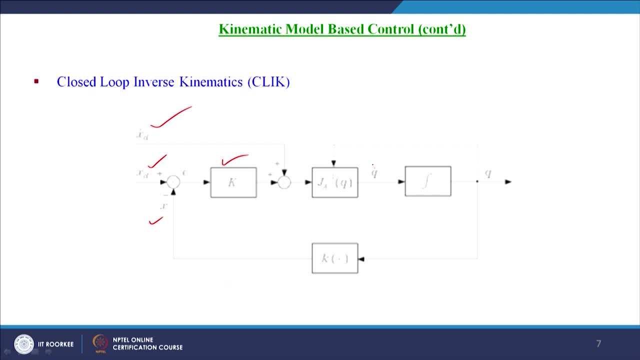 that it is finally, q dot is equal to J A pseudo inverse J A inverse this one into x d dot plus k e. And then q is obtained by the numerical integration of the joint velocity and this portion is nothing, but the forward kinematics given the joint angle obtained the actual tip trajectory. That is compared to get the error and this iteration process. 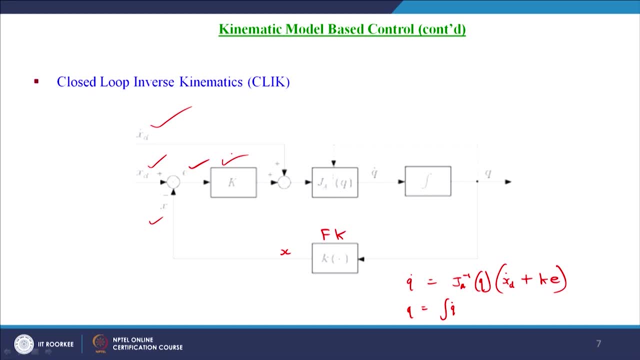 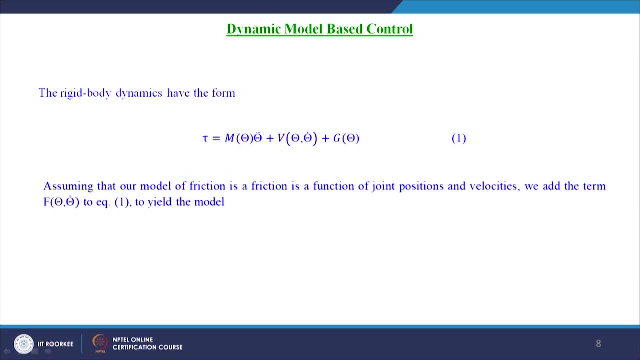 continuous till we reach the final trajectory. Now, coming to the dynamic model based control scheme the rigid body dynamics is given by tau equal to m of theta into theta double dot plus v of theta into theta dot plus g of theta. So, this will be like this v of theta into theta dot multiplied by theta dot plus g of theta where m of theta is called inertia matrix which is of size n cross n. 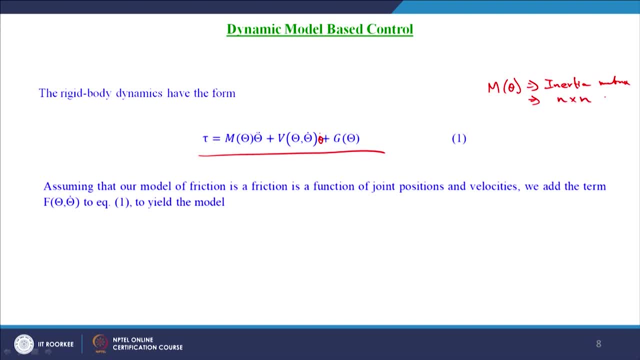 . Where n is the degrees of freedom of the manipulator and v of theta comma theta dot is given by 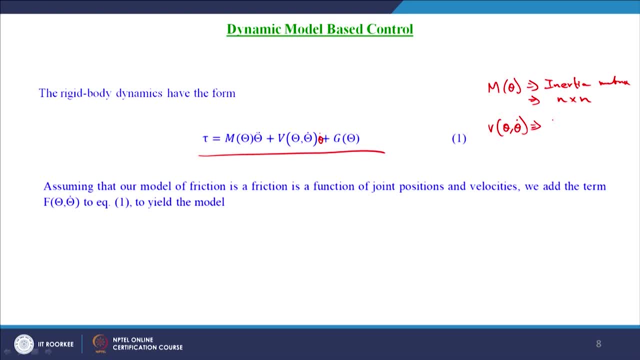 it is called as the matrix which involves the centrifugal and Coriolis effects. Centrifugal and Coriolis effects this is also of size n. . The inertia matrix depends on only the joint angle not the joint velocity, whereas this matrix which covers the centrifugal and Coriolis effects the one which depends on both joint angle as well as the joint velocity. And finally, G of theta is the gravity vector of size n cross 1. . 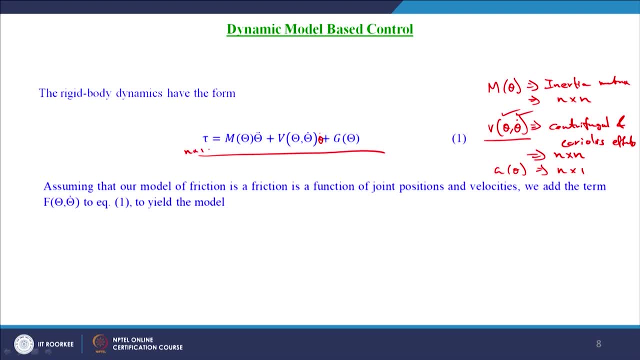 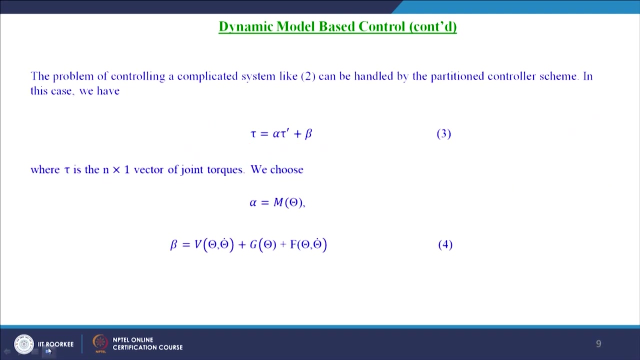 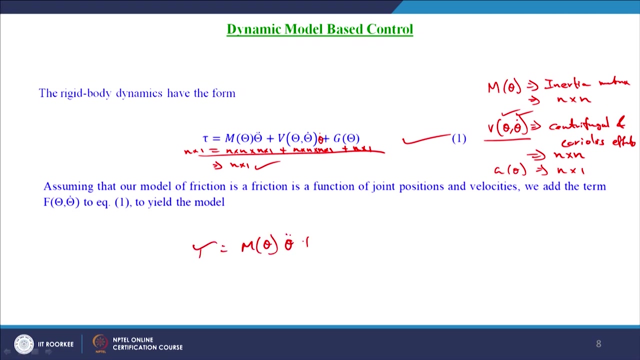 Thus, the left hand side will be n cross 1 which is equal to n cross n multiplied by n cross 1 plus n cross n multiplied by n cross 1 plus n cross 1 eventually gives n cross 1 which is the joint torque vector of size n cross 1. Assuming that our model of friction is a function of joint positions and velocity, we add that term which is f of theta comma theta dot to equation 1. So, that the model we obtain is will be tau equal to m of theta theta double dot plus v of theta comma theta dot into theta dot plus g of theta plus f of theta comma theta dot. 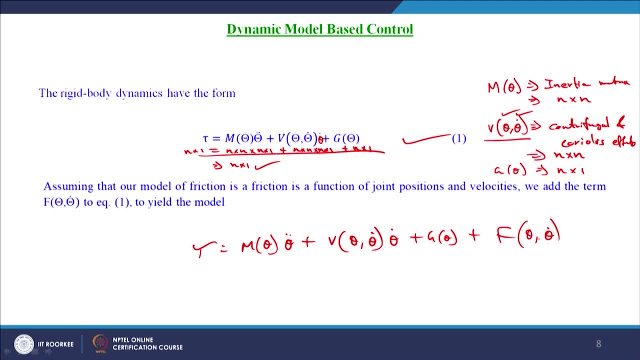 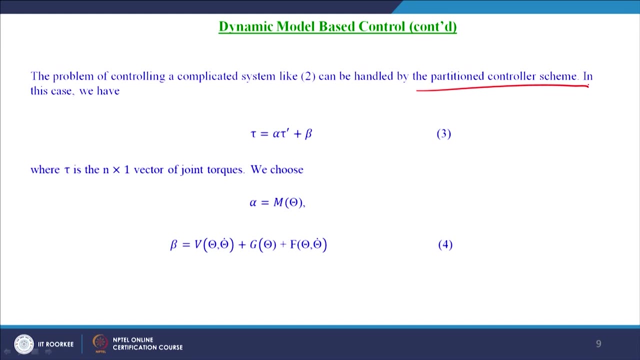 So, the problem of controlling such a complicated system given by say equation 2 can be handled by partition control scheme. So, the partition control scheme can be modeled in such a way that tau equal to alpha tau dash plus beta. . . Where, tau is the n cross 1 or 1 cross n cross 1 vector of joint torques and here we choose from this model we choose alpha equal to inertia matrix m of theta and beta is the rest of that dynamic equation which is v of theta comma theta dot into theta dot plus g of theta plus f of theta comma theta dot. . 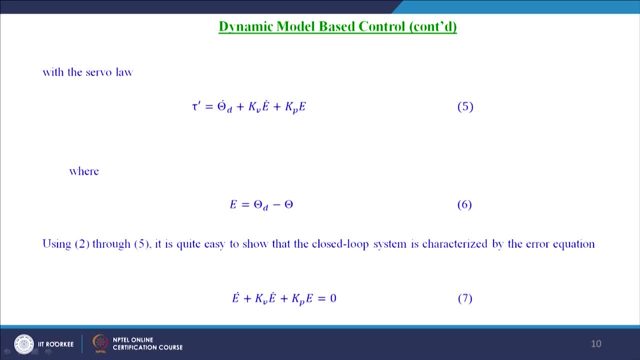 With the servo law, we have the servo law considered. So, that the feedback from both velocity of the joint trajectory also the position of the joint trajectory error is considered in the servo law. So, that tau dash is the servo law given by tau dash equal 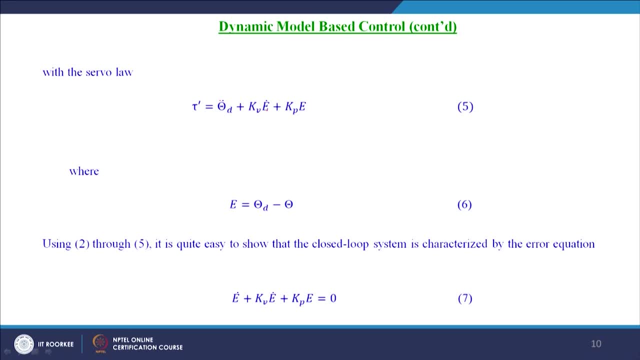 to theta d double dot plus k v e dot plus k p into error. . . 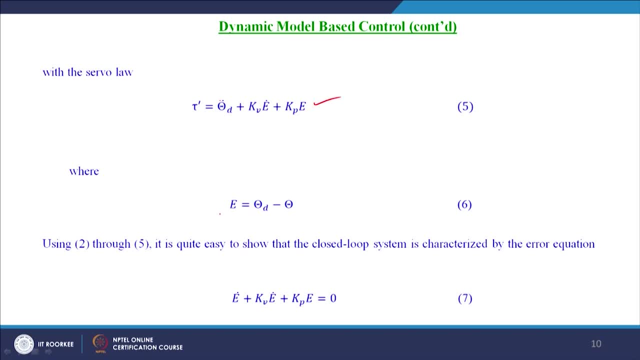 Here comes a ment aquela نموή E, where the error E is given by the discrepancy between the desired joint angle and the actual joint angle. . 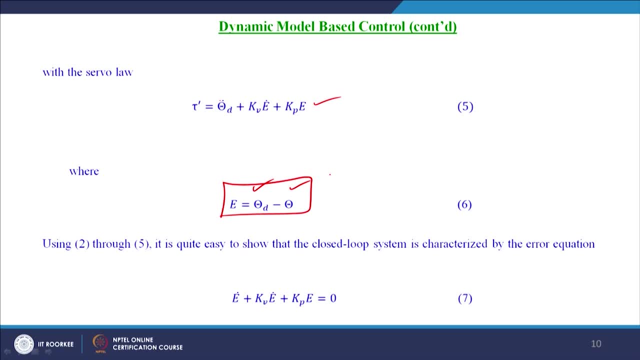 So, using the equations from 2 till 6 or till 5, it is quite easy to show that the closed loop system is characterized by the error equation, second order error equation which is given by E double dot plus k v e dot. . . . E double dot plus k v e dot plus k p into error. So, thisasia lower browser, k v is 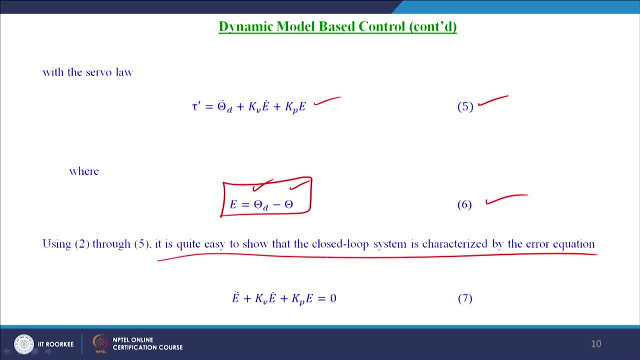 same, what is the error in angry, w is d u by u n m r, d z is a lower vector, v is d z drop by d u, so, straw into d u by d u by d z'th, double underestimate e c t t R of the работ is e dot atol, because we have to e dot plus k p into error is equal to 0. So, this is the second order error dynamic equation 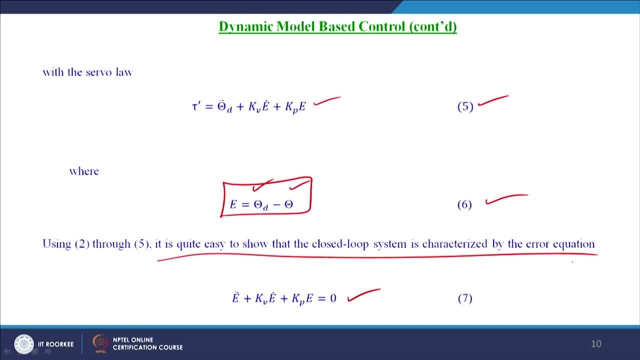 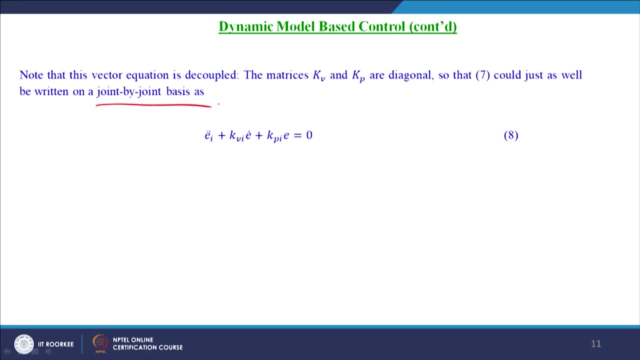 which assures that as a time tends to infinity the error tends to 0. Note this the matrices k v and k p are diagonal. So, for a joint by joint basis for the joint i that error dynamic equation can be written as E i double dot plus k v i E i E dot plus k p i into E is equal to 0 which is equation number 8. 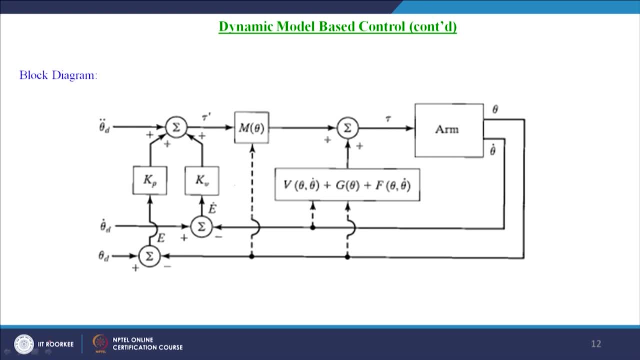 Now, coming to the block diagram explaining or schematically representing the dynamic model based control scheme is shown here where we give the joint trajectories as the input and we are computing the joint torque based on the servo part here based on the servo law that is given by tau dash ok. So, that the servo law is here which takes care of the actual position of the robotic system and this is the portion which is the model based portion. So, we have the dynamic model here when we add this inertia matrix with this the rest of this portion, we get the tau which is basically the dynamic model of the system thus this portion of the block diagram is called model portion. 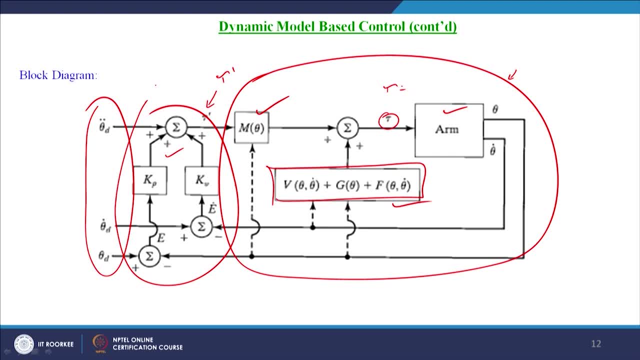 portion is called servo portion. Thus it has been partitioned into servo law and the model based law because the dynamic model is getting involved here. So, now the input here is the joint trajectories and the output here is the joint torque. This is the control part and giving the joint torque to the robotic arm how we get the joint angle joint velocity. Because we need to have the error coming out from the servo law which will be happening because of the discrepancy between the desired trajectory and the actual trajectory. 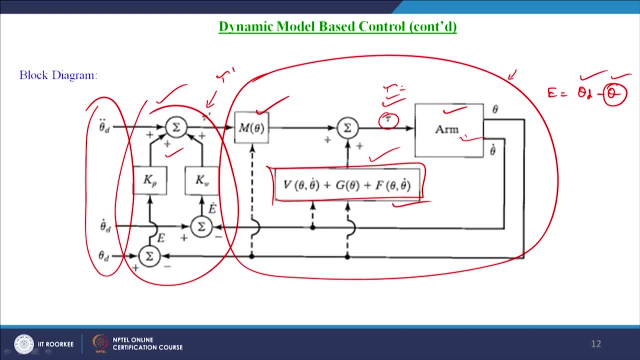 So, we need to know the actual trajectory that is done by this portion which is here the simulation is happening which is giving the joint torque to the arm robot arm we are getting the joint velocity that is tau equal to say m of theta theta double dot plus v of theta comma theta dot. So, tau we know because we are giving that as the input. So, theta m of theta into theta double dot is equal to tau minus say the rest of the portion is say x and theta double dot equal to m of theta. So, m of theta inverse tau minus x. So, theta dot will be obtained now by integration of this acceleration further theta which is joint angle will be obtained by the integration of joint velocity. So, this is how we obtain the joint actual trajectories from the manipulator given the joint torque. . . 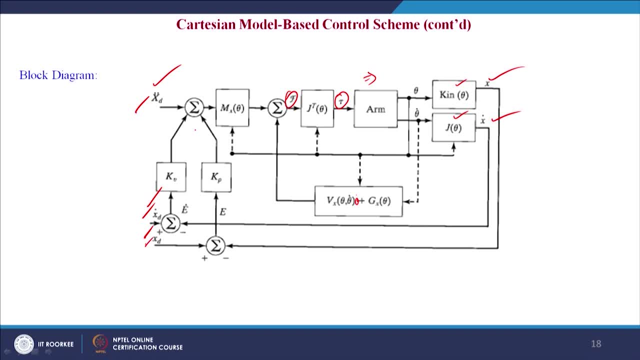 , in order to obtain the actual in order to obtain the error. So, that we could be able to compute the joint torque through J transpose F with this control law we could be able to get the actual joint torque and from that we could be able to obtain the joint angle through forward kinematics and inverse kinematics we could be able to forward kinematics 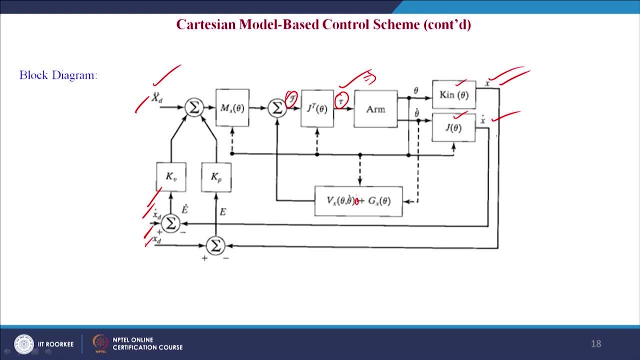 and differential kinematics we could be able to get the position and velocity of the manipulator. . 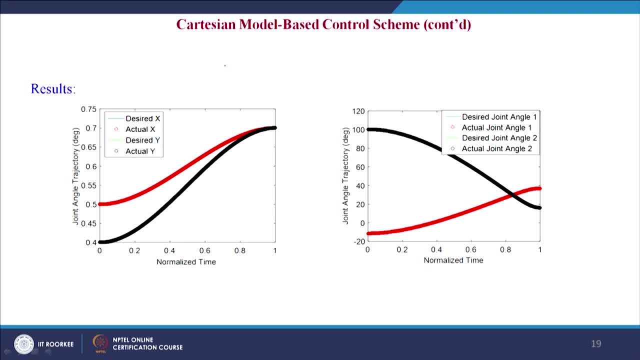 And similarly for the 2 R planar manipulator case we could able to obtain the decide trajectories this is basically in effect position which is in centimeter and this is also the joint angle trajectory this is correct. . 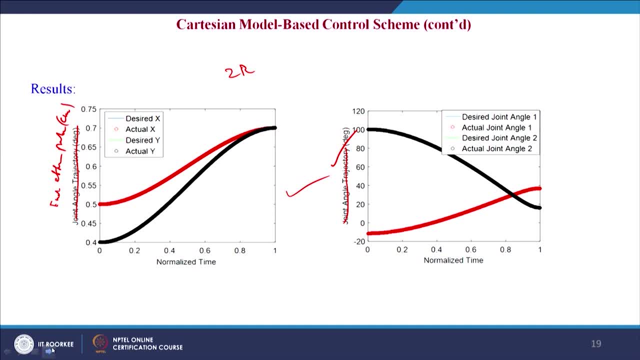 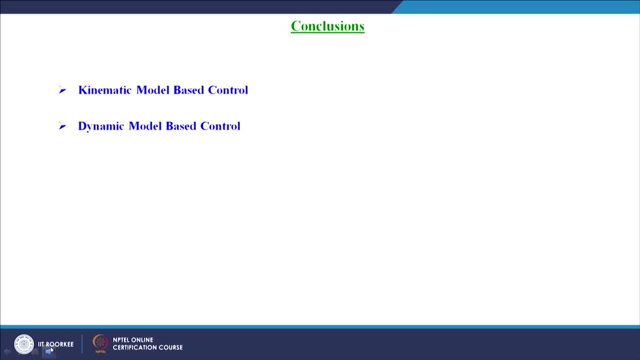 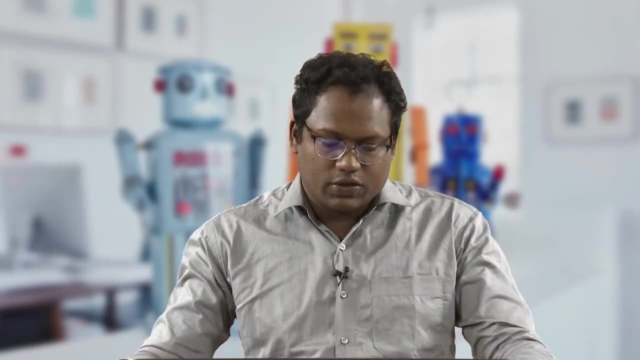 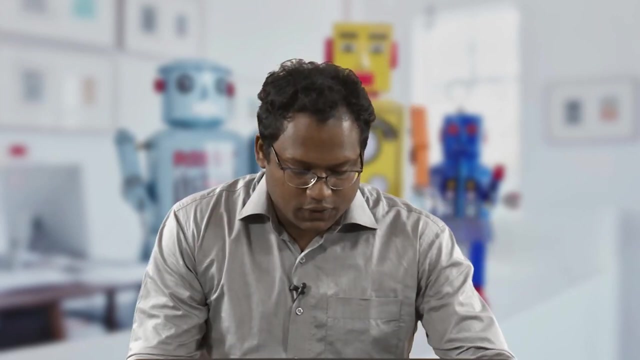 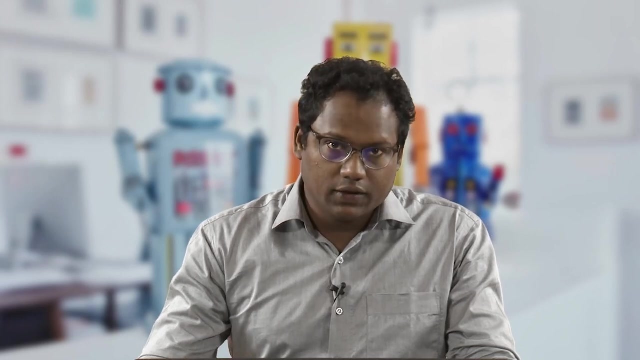 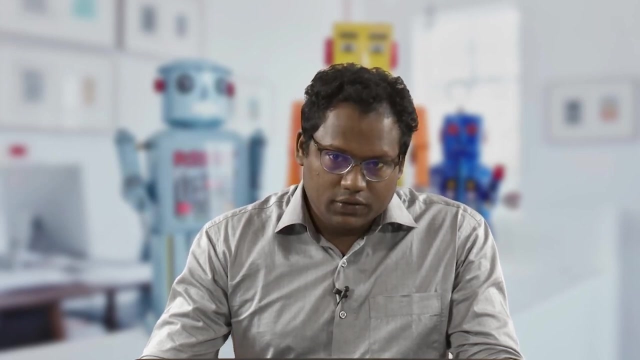 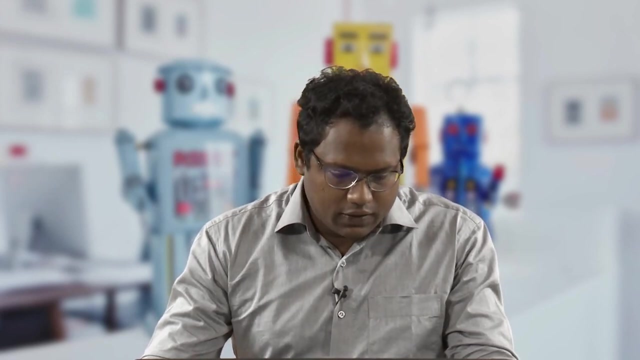 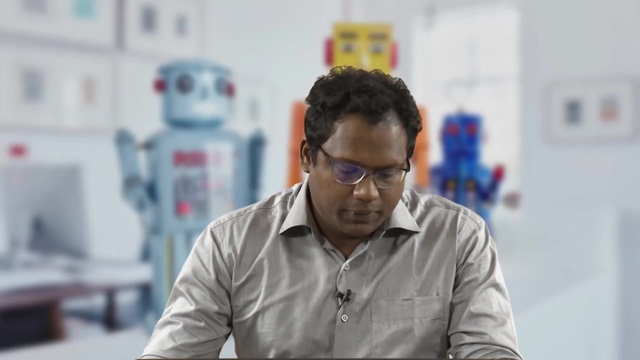 This joint angle trajectories now coming to the final conclusion part. So, we just finished with this Cartesian based control and now we conclude this session in such a way that in this lecture we have simulated both the kinematic model based control scheme and the dynamic based control scheme. . . So, we have in this lecture we have seen the basic definitions of kinematics, dynamics and the types of kinematics the classification of kinematics and the classification of dynamics in this lecture. And then we entered into the model based control scheme with which is further classified into kinematics model based control scheme and dynamics model based control scheme. . In the kinematics model based control scheme. . 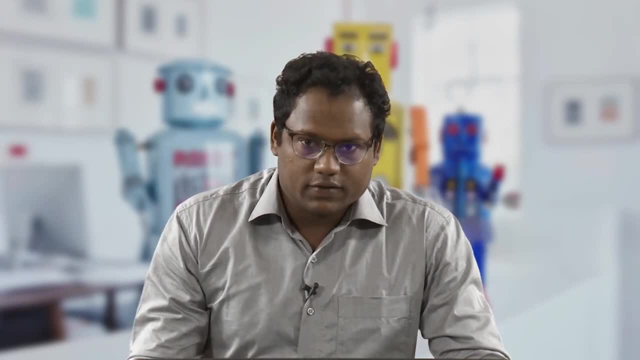 kinematics model based control scheme, we have seen the CLIK that is closed loop inverse kinematics showing the error dynamic equation which is the first order error dynamic equation. 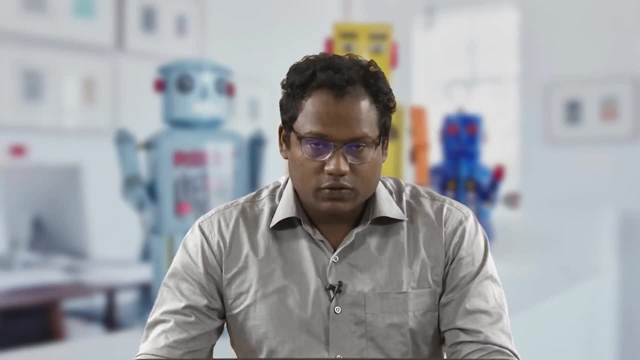 Whereas, for the dynamics based control scheme, we have seen the inverse dynamics based control 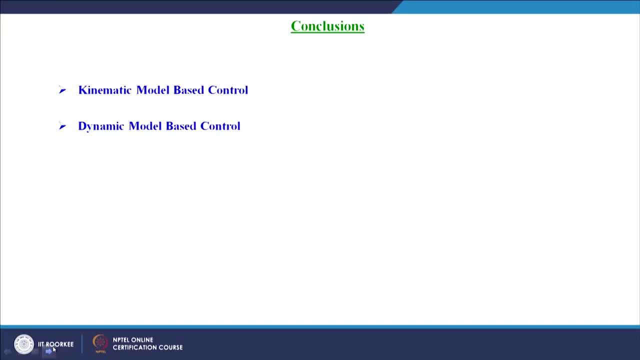 scheme which is the model dynamic model based control scheme which is involving partition control scheme and also we have done that through joint space control and Cartesian space control. Thus in this lecture we have seen the control scheme of manipulators based 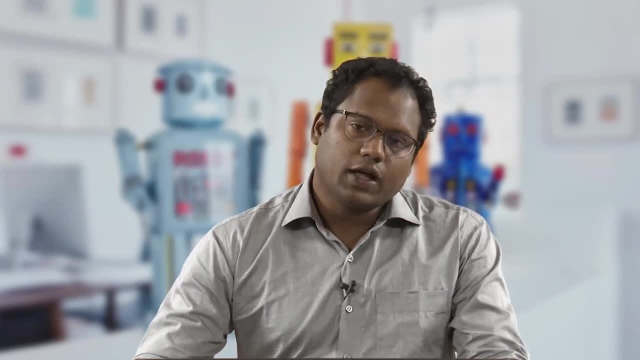 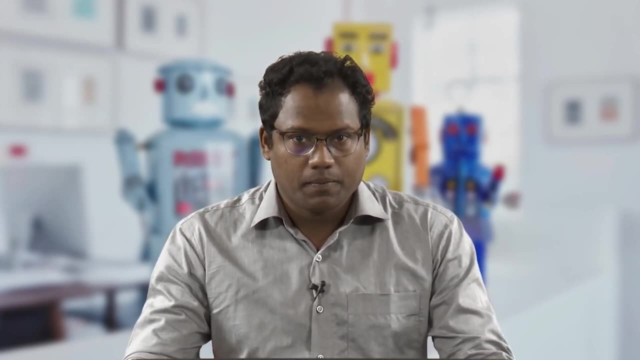 on the model based control. The model based control has been classified into kinematics model based control scheme and dynamics model based control scheme. 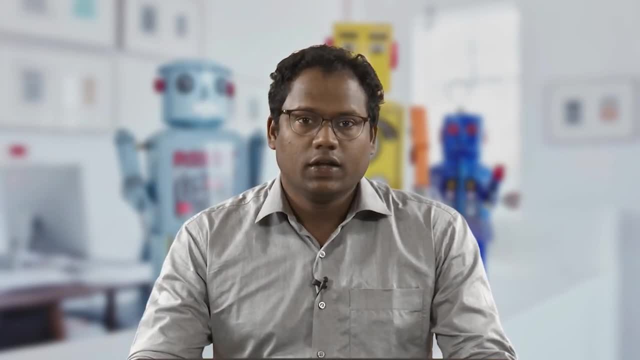 The kinematics model based control scheme what we have seen in our lecture is closed